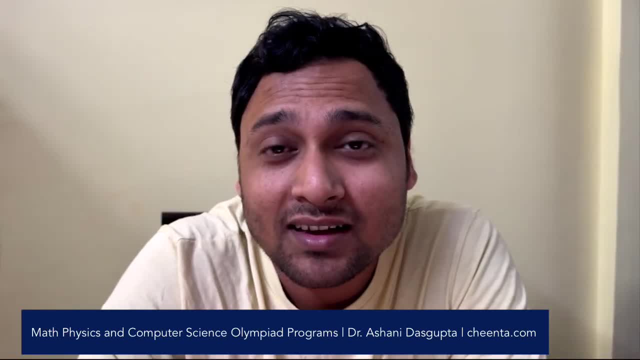 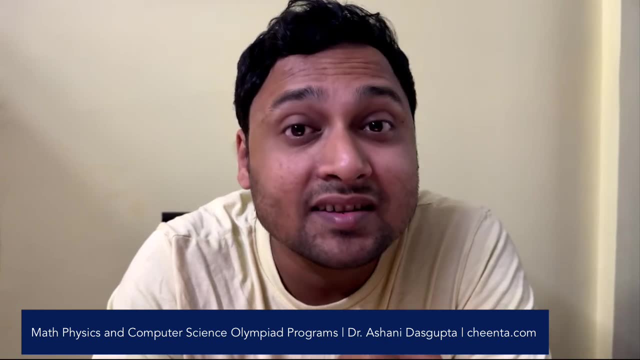 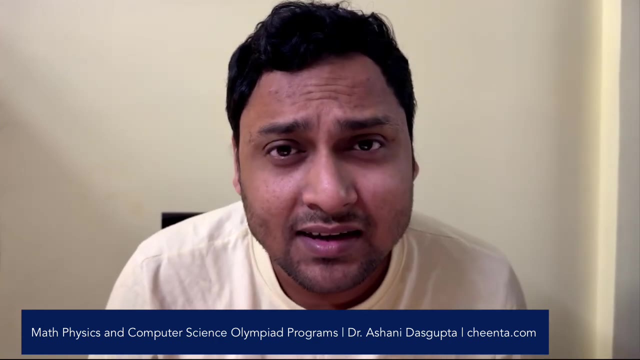 Hello everyone, this is Ashwani from Jeddahcom. In this particular video, we will talk about books and resources for mathematics, physics and computer science- Stuff that we use regularly in our Olympiad and research programs, especially for elementary school students and middle school students. 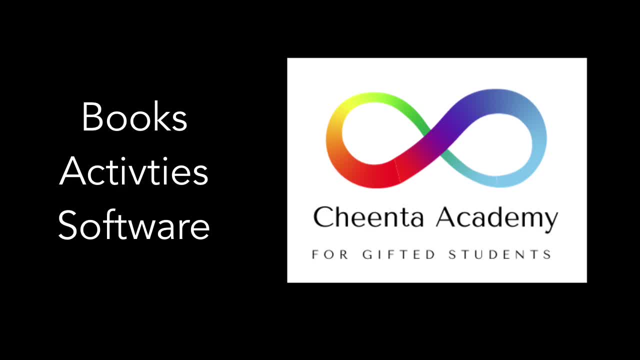 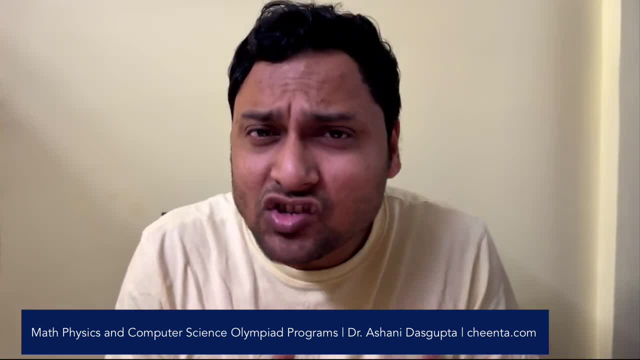 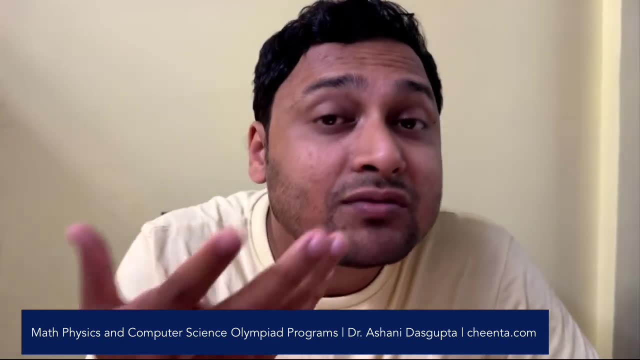 We have been using these tools for quite some time- the last 13 years- And you can check the link in the description for our courses. But even if you are not enrolled in one of our courses, you can use these at your home And I think they will be very useful. 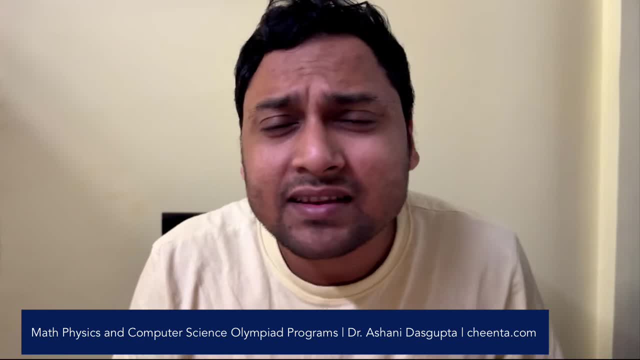 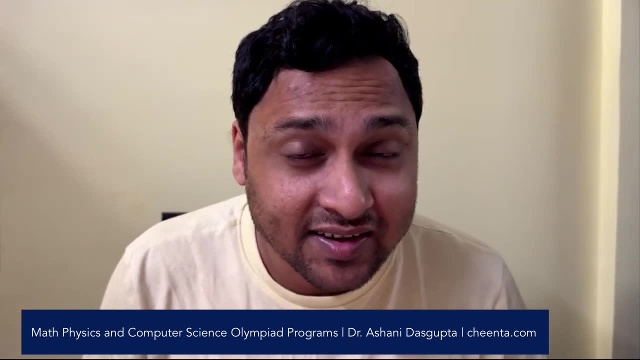 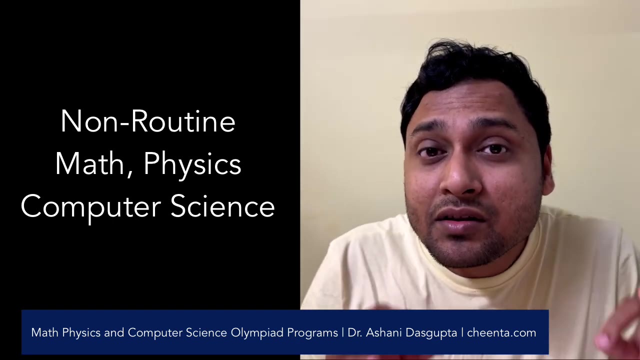 So let's get started, And we will start with elementary school students. But the kids are just starting out with their journey in non-routine mathematics, physics or computer science. When we say non-routine mathematics, what we mean is problems that make you think. 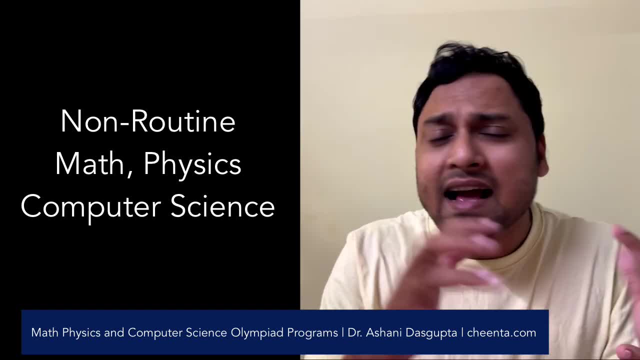 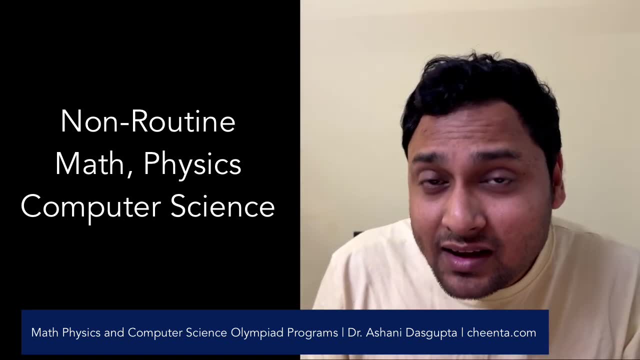 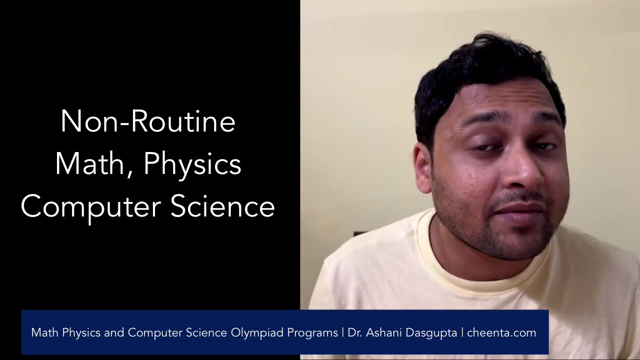 These problems you cannot just plug in a formula and just solve it over 30-40 seconds or one minute. They are not repetitive in nature. Instead they actually appeal to the intellect, The intellectual capacity of the child. We call these type of mathematics slow math or slow physics, or slow computer science, depending on what you are doing. 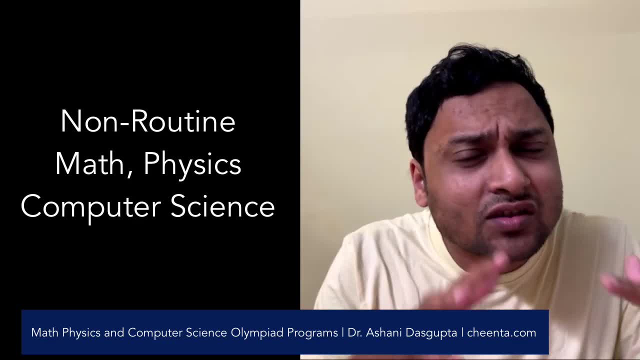 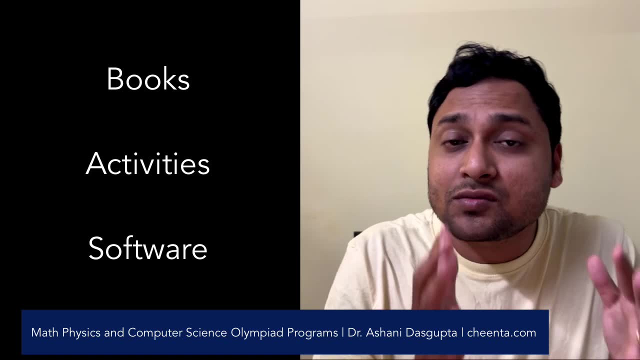 Now there are a lot of resources which focus on this type of mathematical sciences. I have divided broadly into three categories these resources. The first one, books that you can have. The second one are the set of activities that you can actually use. 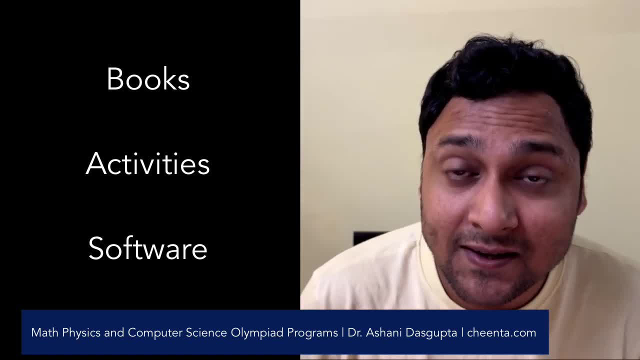 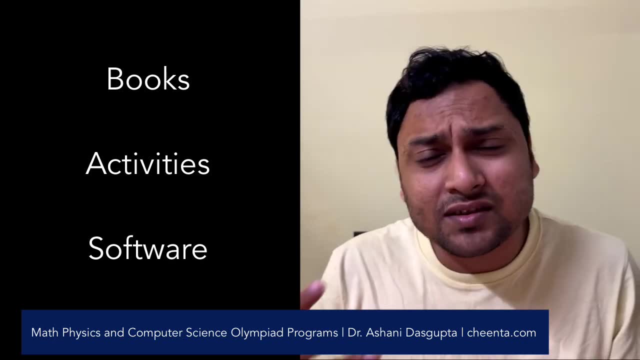 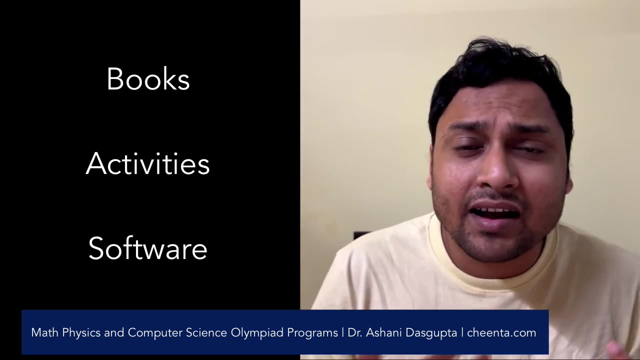 And the third one is the sort of softwares and technologies that you can use at Chinda in our mathematics career programs. We actually use all three of them. You also use the same in physics and computer science, but very easy And you can use them in at your home when you are training or helping. And that also actually applies to the training that you you're involved with. 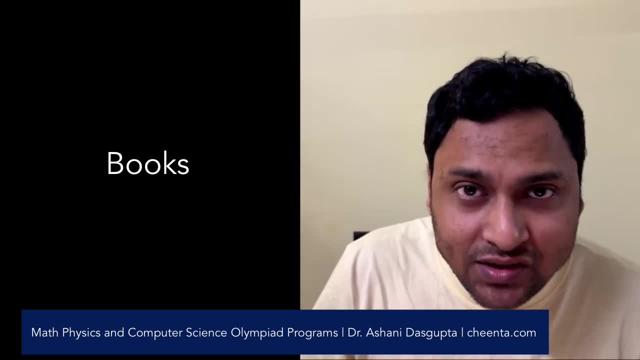 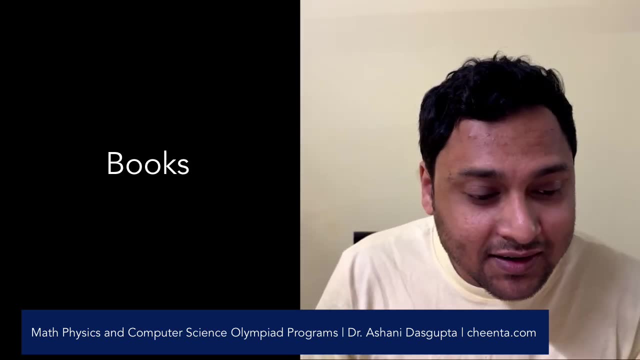 Your own child. So let's talk about the books. So to avoid making mistakes, I have actually written it down in her place. These are all russian authors There. many face is much a. This is what Alight: Get a book for seven minutes. 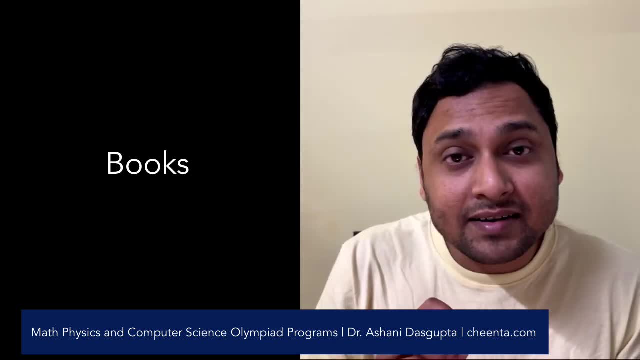 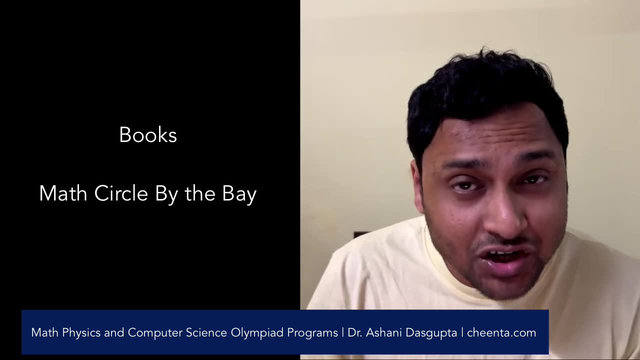 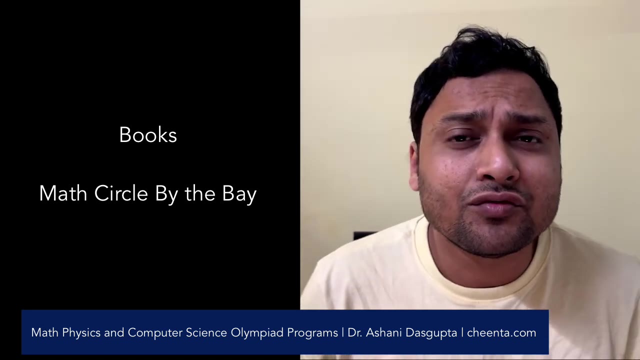 elementary school students. the first book that i will recommend is math circle by the bay, topics for grades one to five. this is by zakharavish and there are some more authors. it's a very beautiful book written by mathematicians who work in the berkeley. 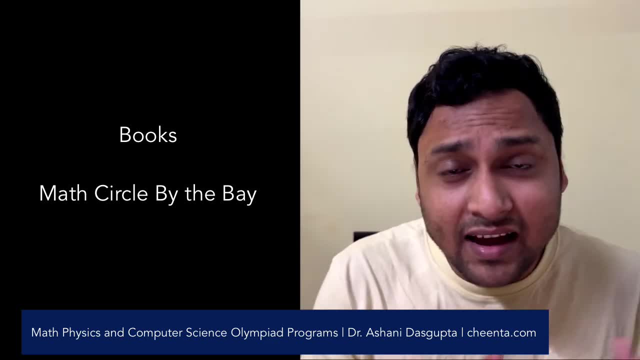 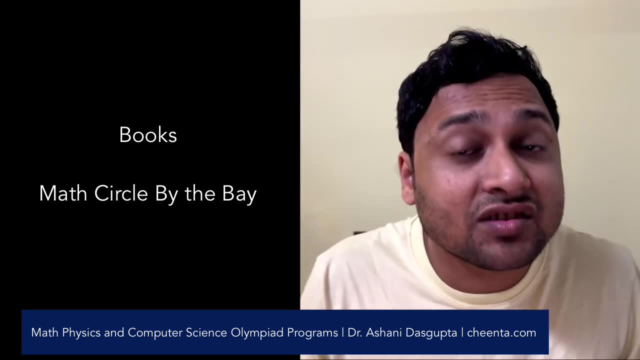 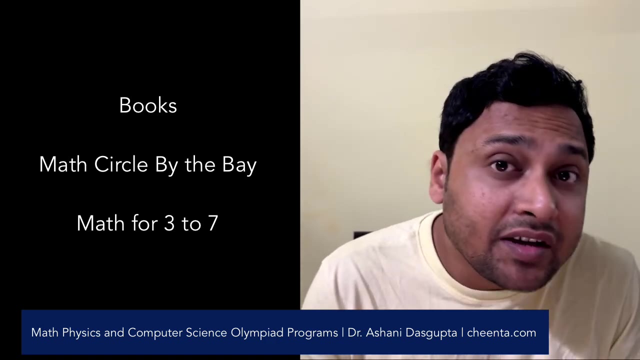 math circle program in the california region of united states. it's a fantastic book. it has activities and problems that motivates the child to think. there is another book of a similar flavor. it's called math from three to seven. math from three to seven. this is again a math circle for 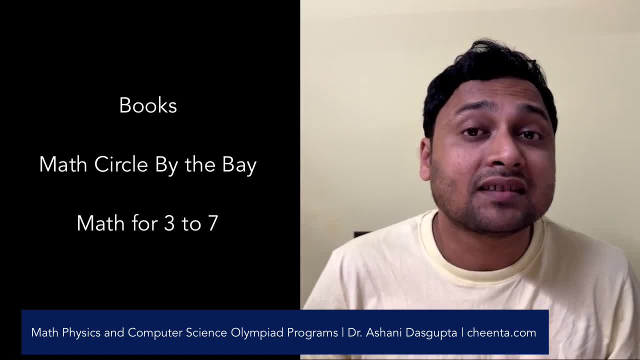 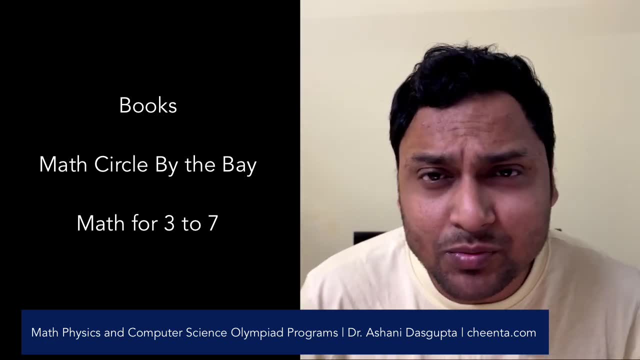 preschoolers. this is written by someone called zovonkin so you can google that app. i also put a link of that in the description section. you can also check that out. all of the names rates are given in the description section of this book and the link is in the description. 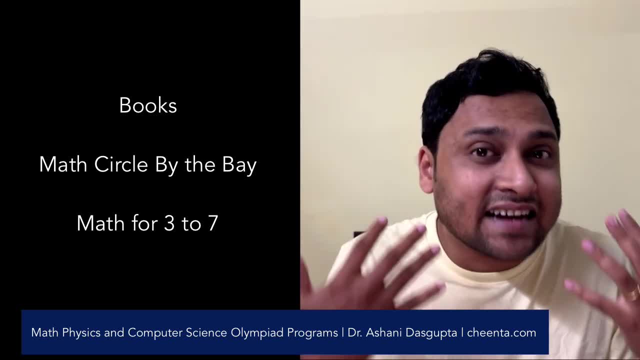 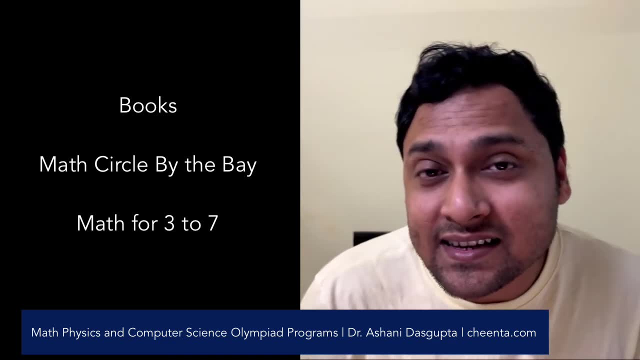 you can also check that out- all of the names we have in the description section of this book and there this particular book is like a diary of math circles, where the coordinator or the faculty works with three or four kids and they, they together do problems and activities which make you. 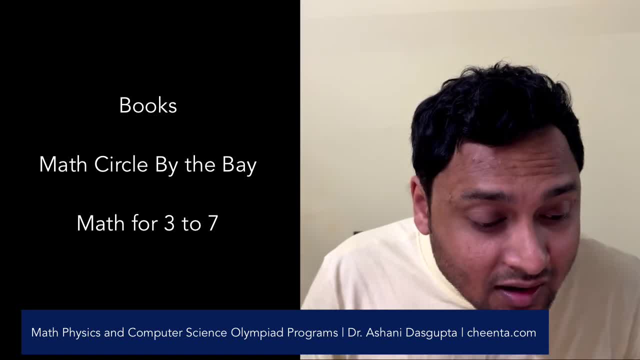 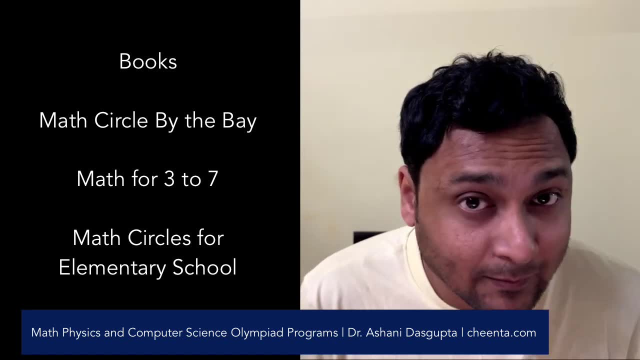 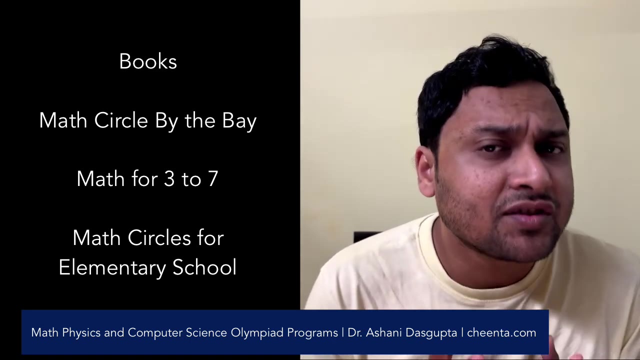 think: okay, that's the second one. the third one is called math circles for elementary school students. this is by natasha robs rostkovskaya, again a book of similar flavor. what we try to stress at the elementary school level is that you do not really need to memorize. 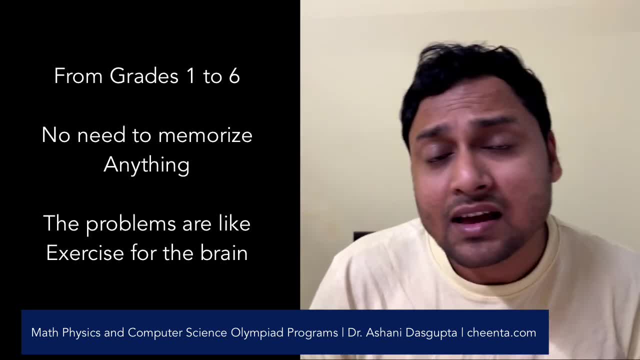 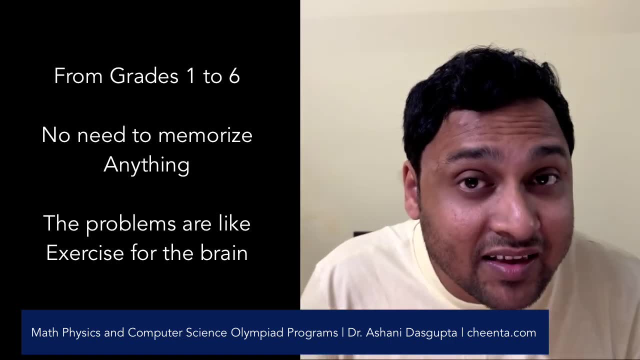 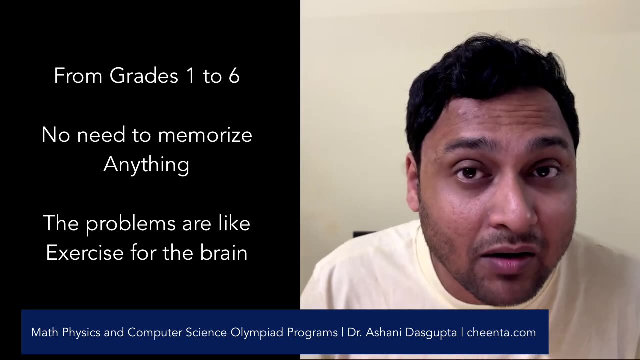 anything. in fact, that's not even suggested. instead, take one problem at a time, try to think, try to spend time with that problem, make some doodles in your notebook, make some small która, communicate with others about the problem, and maybe you forget about the problem entirely after. 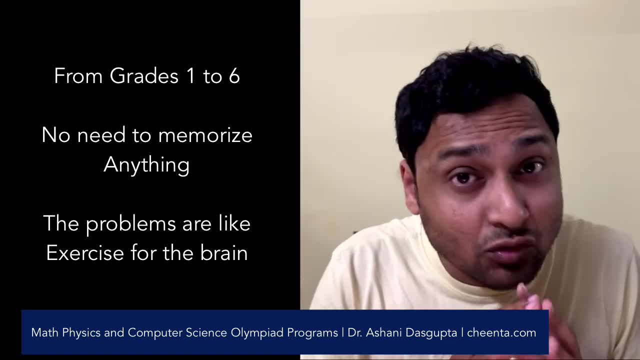 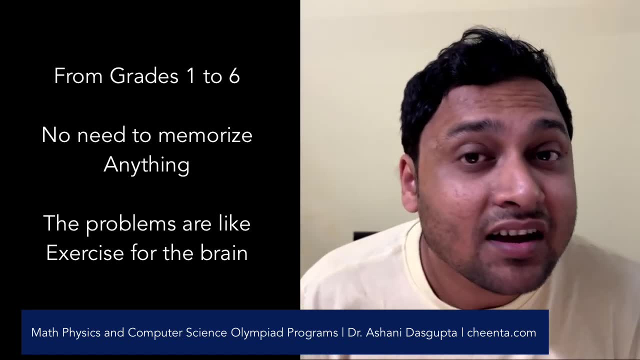 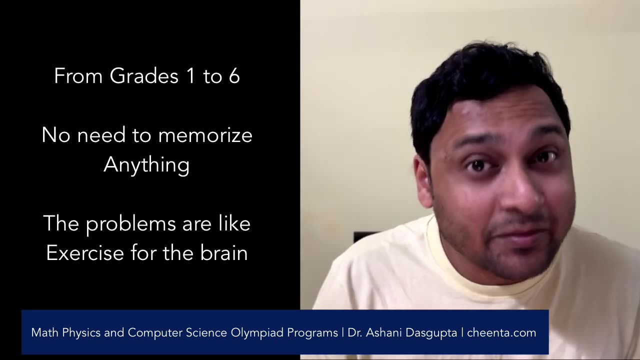 a couple of weeks. children forget things all the time. that's totally fine. you do not need to remember anything. think about these things as exercises for your brain muscles. you don't remember, that's not a problem, but you do it every day. that's the point, okay, so these are the three. 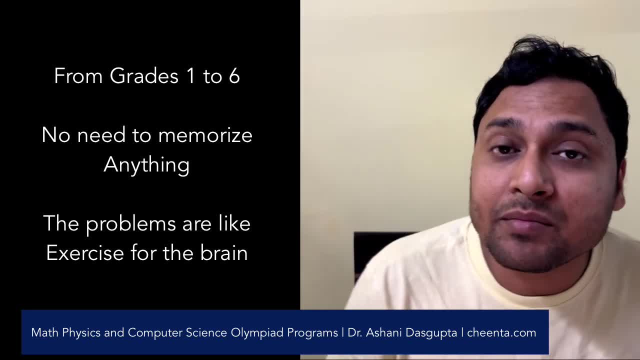 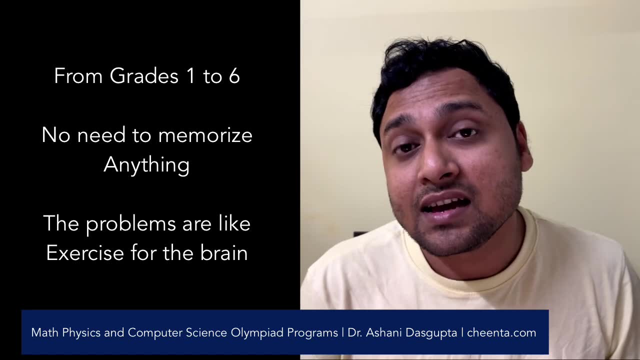 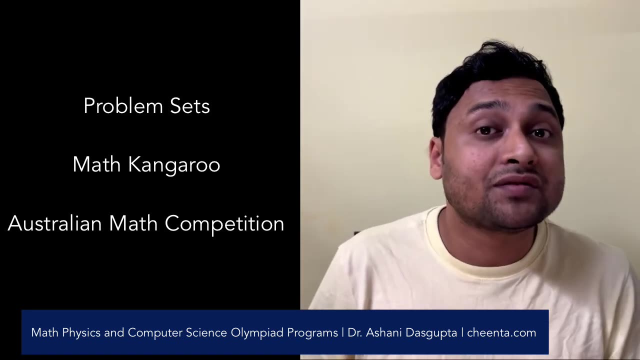 books that we strongly suggest. of course, in our elementary school mathematics olympiad foundation program we use other problem sets and resources as well, so i'll let me tell you a little bit more about those problem sets. for example, we use problems from australian math competition. 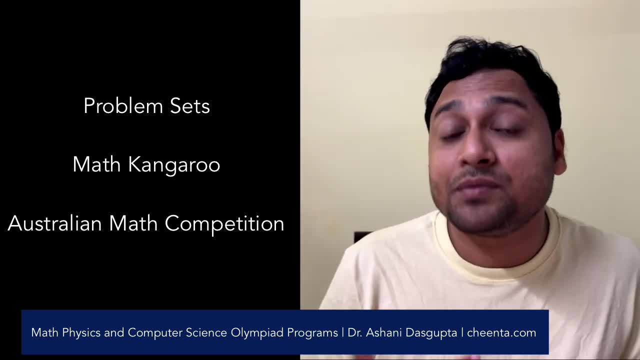 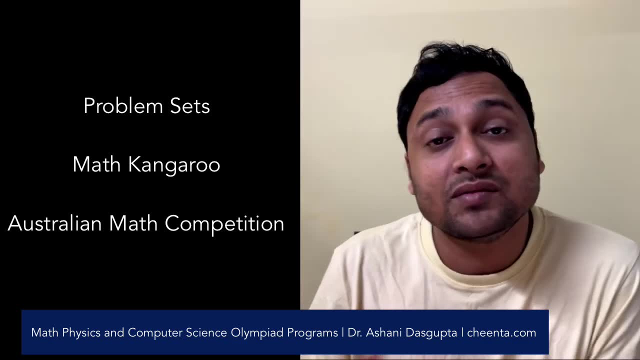 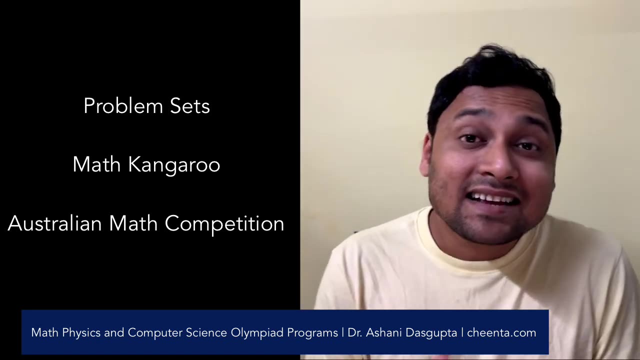 and math kangaroo. these are very nice problems which challenge the mind of the students. so, apart from the books, you should also try to use the problems from these competitions, which are actually interesting for the development of the child. okay, the next set of things that we're going to talk about are activities. so these are very interesting in the 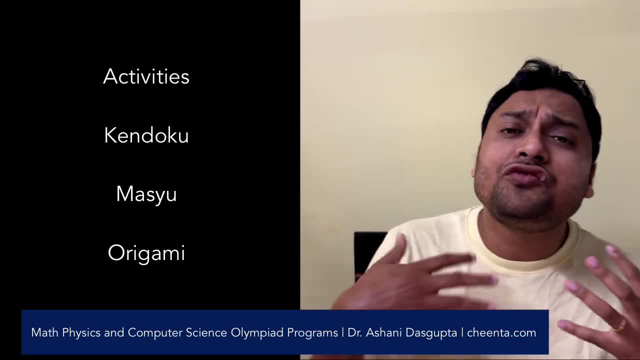 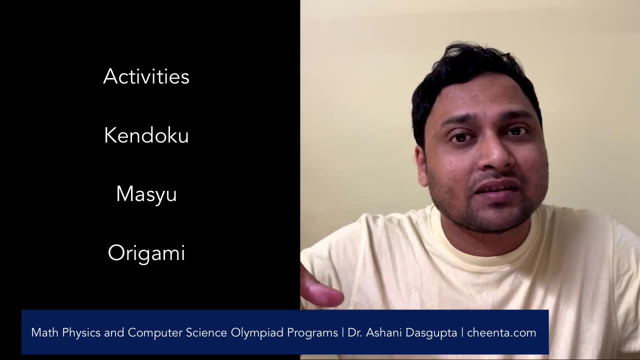 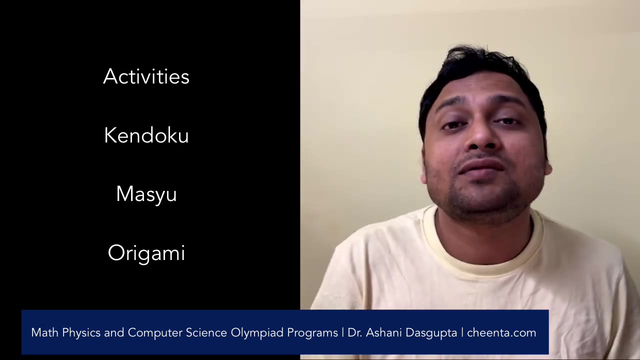 sense they contribute as recess or breaks in the learning style of the child. so maybe the child is talking about geometric patterns, he's thinking about problems and trying to doodle some stuff and he's doing it for some time. but you don't want him to get tired, you don't want to. 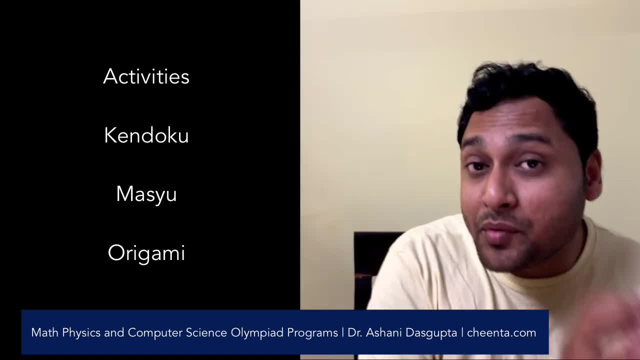 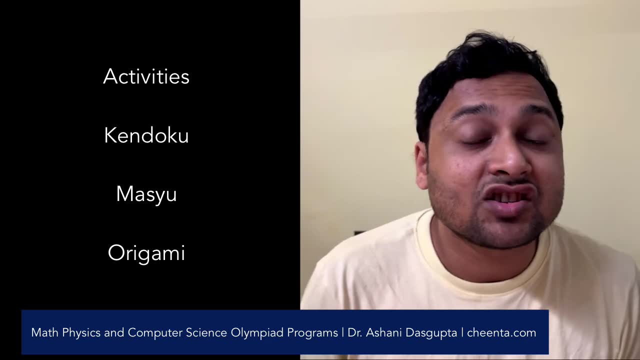 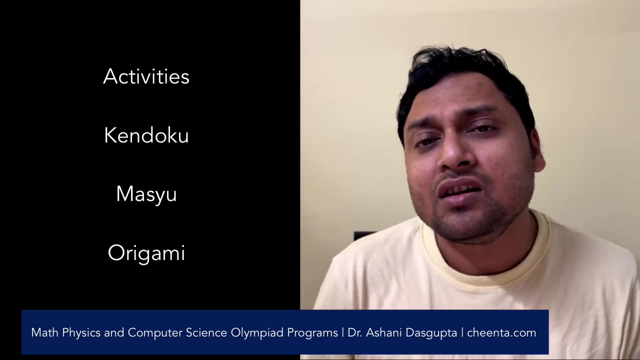 stretch it for too long. so you have to may take a break. you have to let the child take a break as well. so what we can do is you can use activities such as kendaku- kendaku is a japanese game and masiu- masiu is also a similar japanese game, which requires logical thinking, analytical abilities. 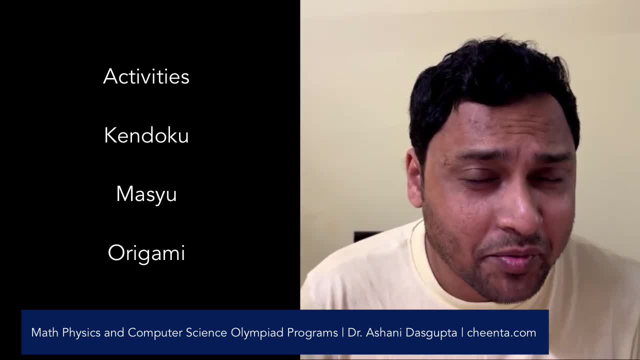 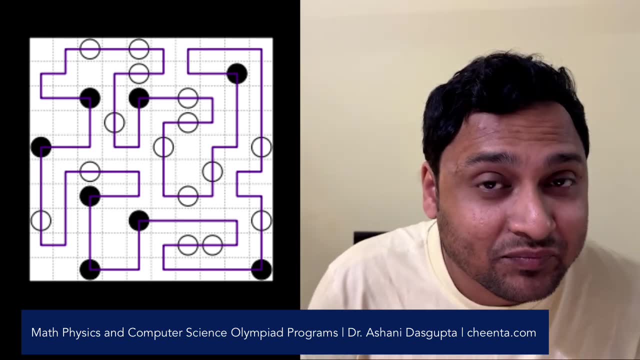 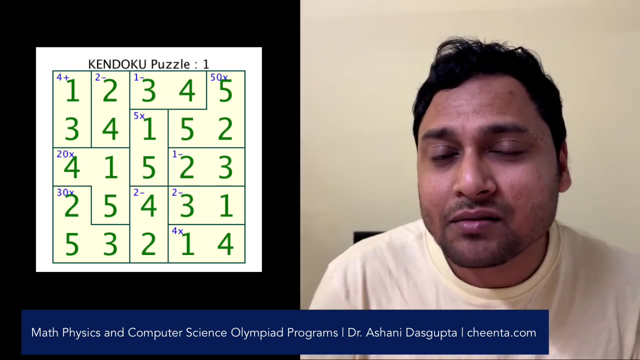 and also the elementary arithmetic operations. these are just simple games which requires you to think mathematically. so we use kendaku, masiu and similar games in the class for like five- ten minutes recess between discussion of concepts. they work really nicely. students actually participate quite a bit. the 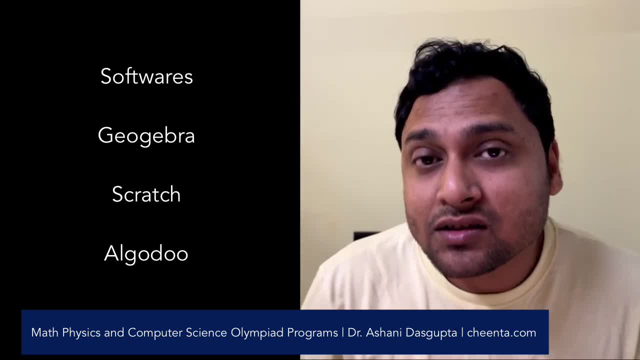 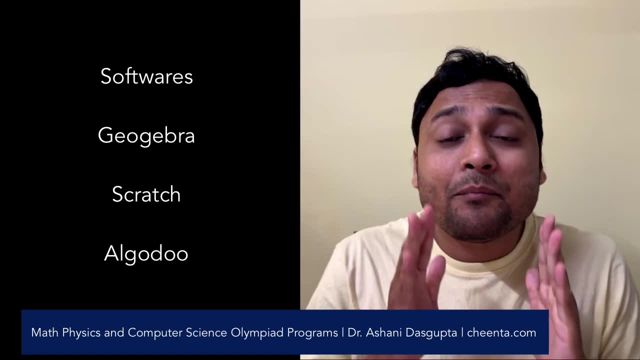 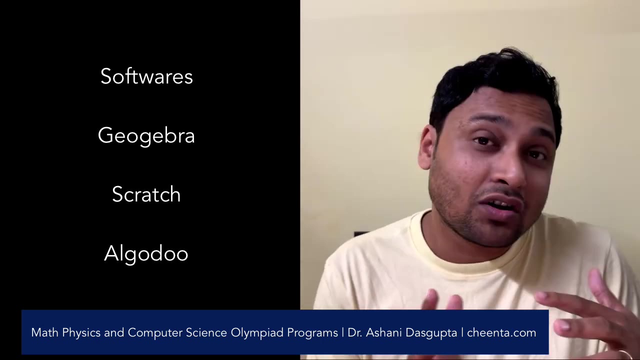 third set of things are softwares. so in this day and age, when we have a ton of softwares which help us to understand the application, it is important that you use some of them. but you should not use too much of softwares. but you should not use like you should not totally reject them as well. so for 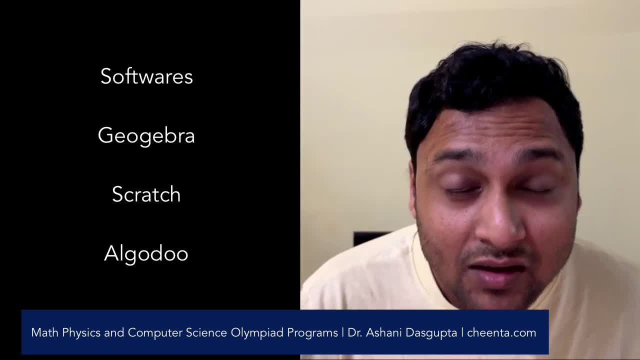 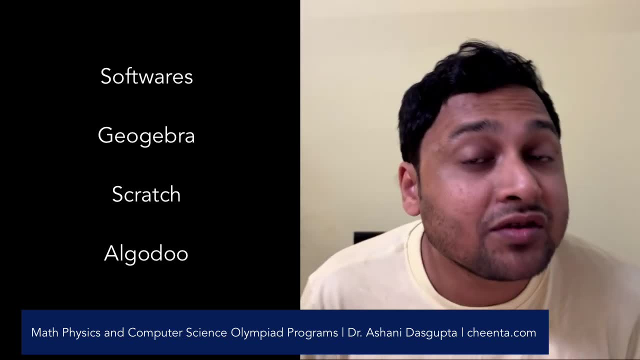 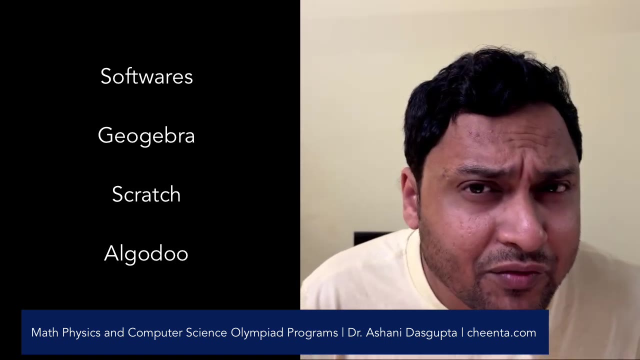 example, in our programs we use something called geogebra, which is a geometry software tool. we use it quite a bit. in the physics program we use tellerium. stellarium is a astronomy related software. you can also use it, available for free. in physics we also use something called algodoo. algodoo is 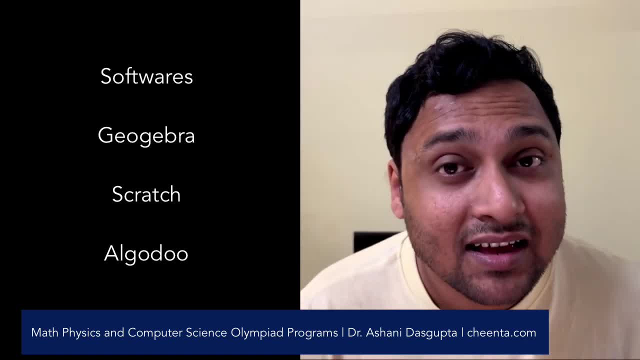 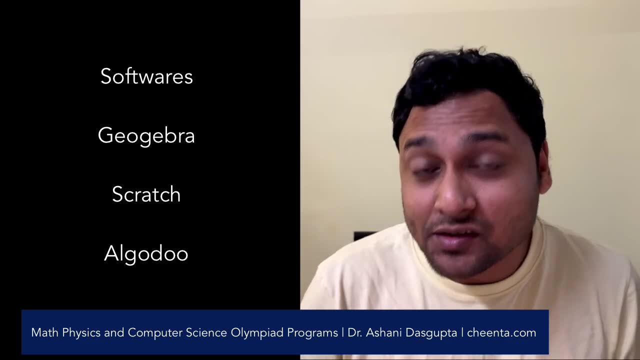 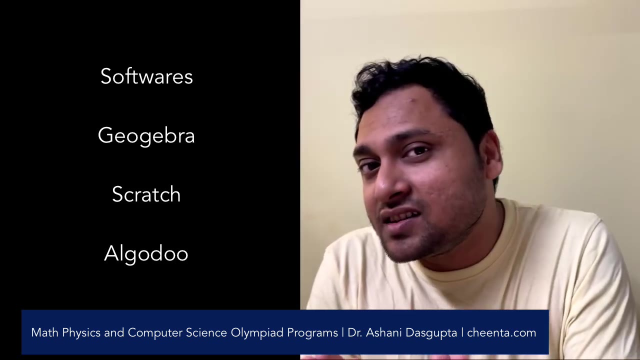 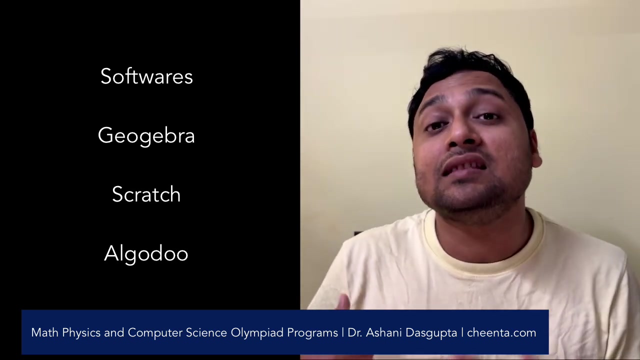 also a physics virtual lab software. this allows the child to play with the different aspects of physics and learn on the way. so these three things- they are extremely important- books, activities and resources, and then we have the software technology. we also have a software called math circles, which is a software that is used by middle school. 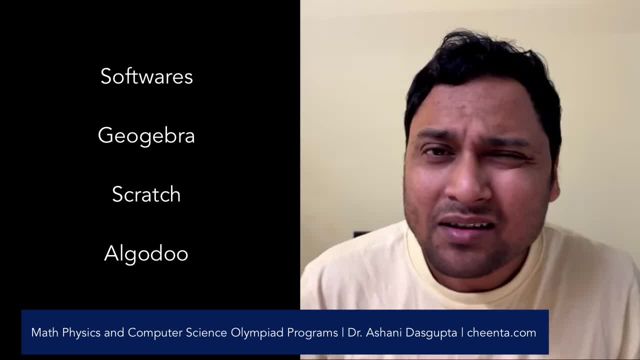 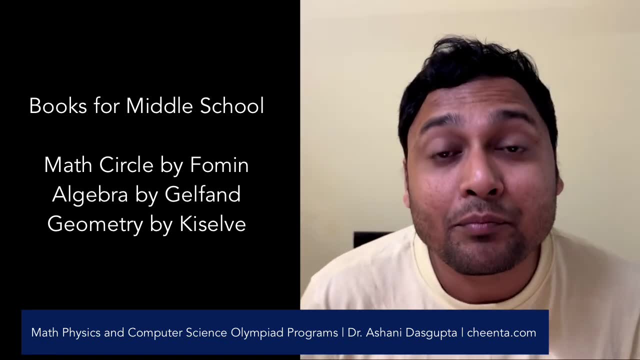 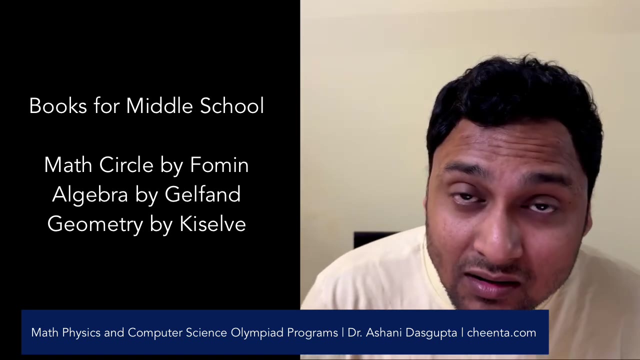 students to write down mathematics in a more professional way. that's another thing that you can explore as well, but it's more for the middle school students. i would also end this particular video by some book suggestions for the middle school students. so the first book is called math. 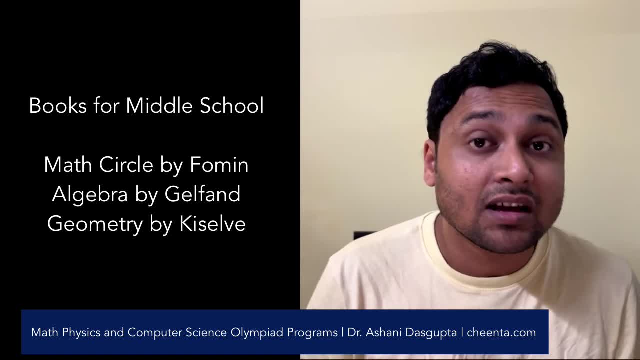 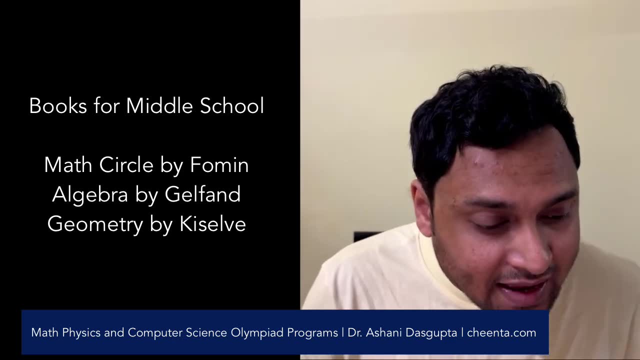 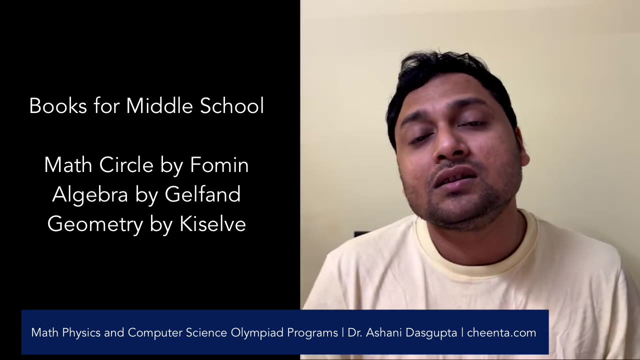 circles by foeman. it's a very beautiful book. you should definitely try the problems in it, especially in year two, but year one in particular if you are just starting out in middle school. then we have algebra by alexander shen and israel- israel gil fund, so this is a very nice book you. 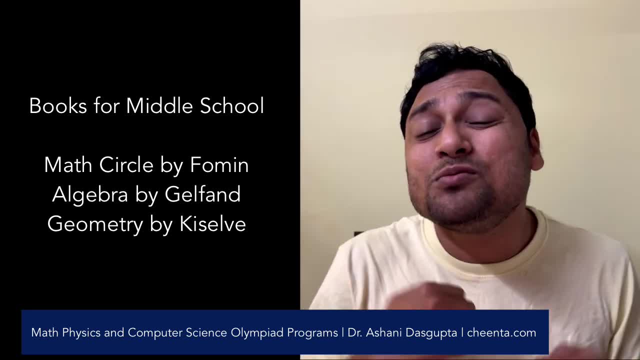 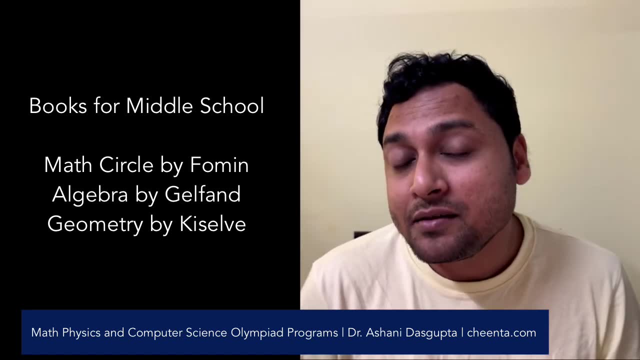 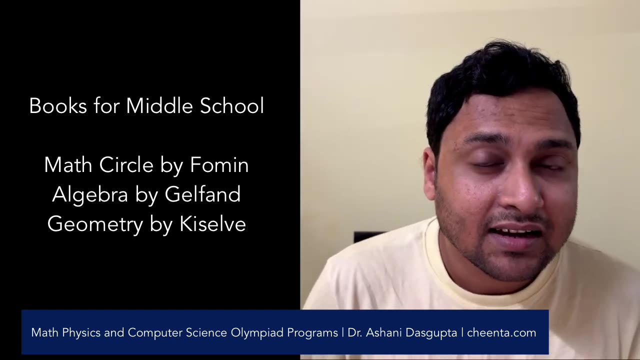 can. it will get you started with algebra, but it will also make you think about the fundamentals of algebra. and the third book is called kiselev's geometry planimetry by alexander givendal. it's also a great book translated into english. it will help you get started with geometry and do interesting. 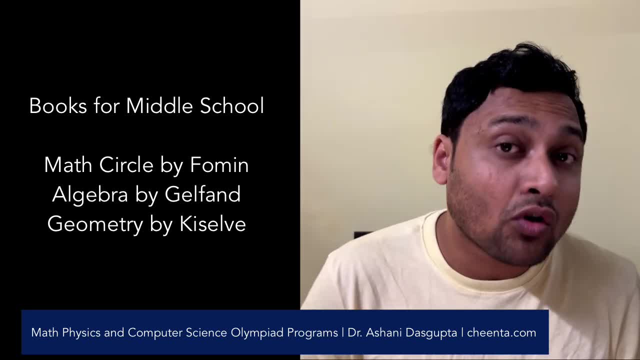 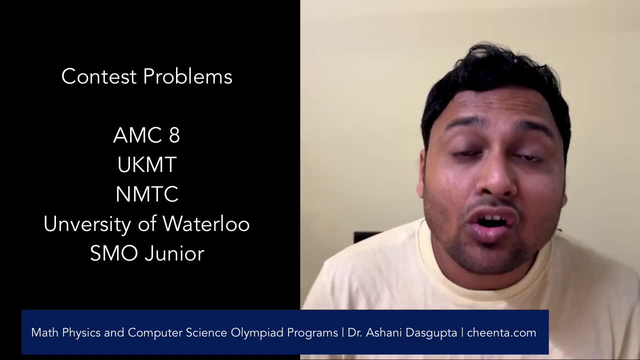 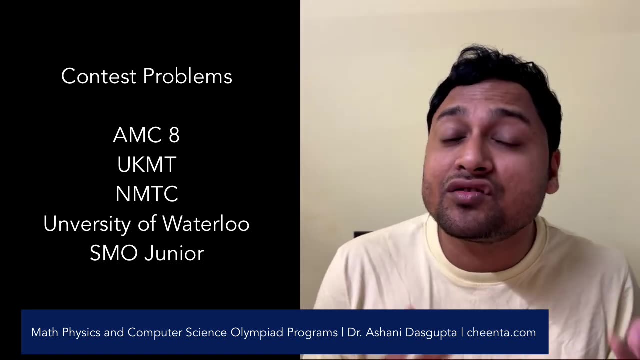 problems in it. in the middle school level we also have some contest suggestions. you can use problems from nntc or amc8, american math competition 8 or ukmt junior or university of waterloo contests. these are excellent contests which have interesting problems. you can try those problems to.